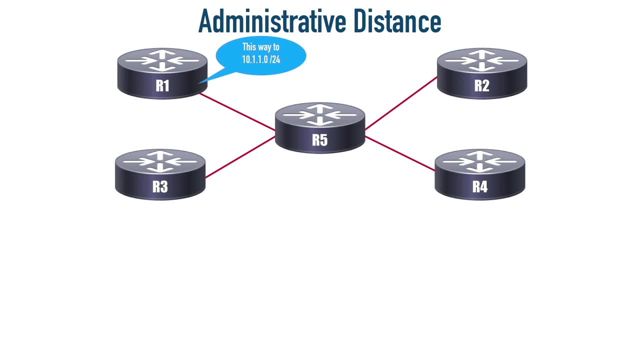 us. hey, this is the way to 10.1.1.0 slash 24.. R2 says here's how to reach that network, R3 says I'll get you there And R4 says here's your ticket to 10.1.1.0 slash 24.. And the question is: who do? 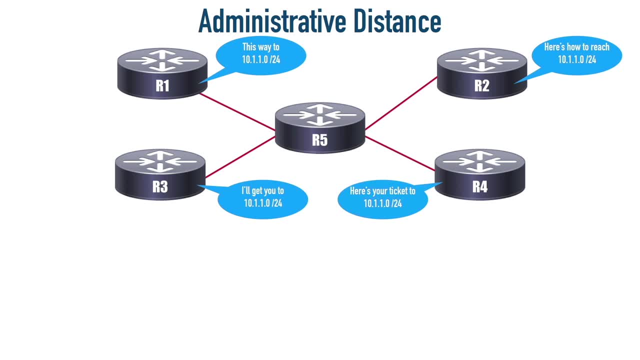 we believe. Well, we have different routing sources. We have different routing sources. We have different sources with different believability. Specifically, some routing sources are more authoritative than others, And the way we measure the believability of a routing source is with something called. 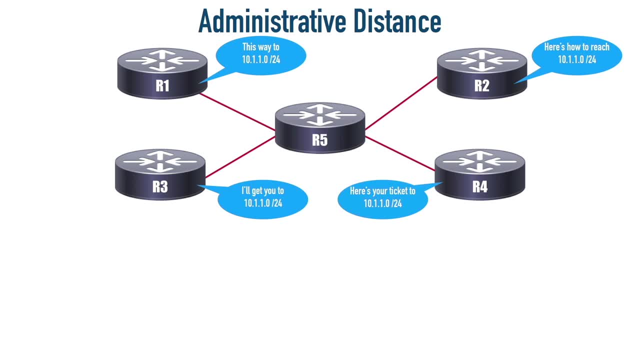 administrative distance, or AD. Let's take a look at some common routing sources and their administrative distances. First, let's consider a directly connected network. It doesn't get more believable than being directly connected to a network, So that has the most believable of all. 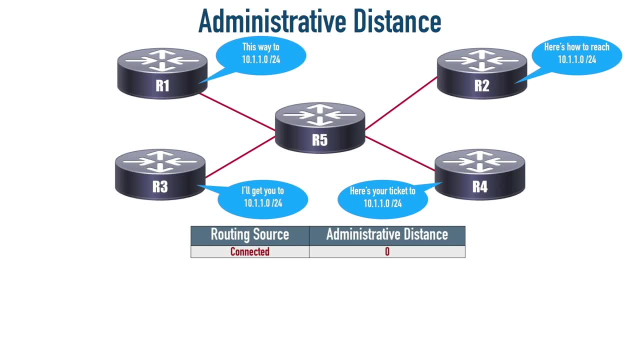 administrative distances a zero, Because lower is more believable. But if we as administrators go in and configure a static route, odds are we know what we're doing and we want that route to be taken into account before any dynamic routing protocols. So by default, a statically configured route has an administrative 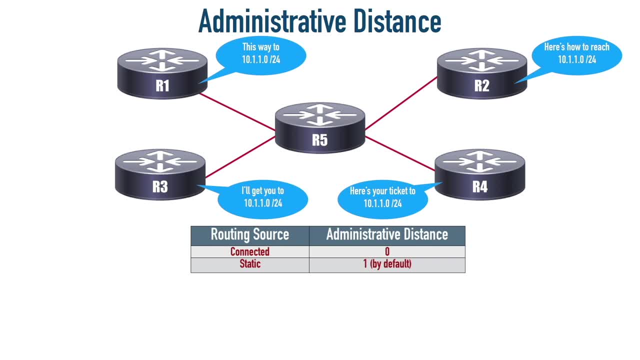 distance of a one. Now notice, I say by default, because we can play some games and do something called a floating static route. We could set a static route with a higher administrative distance, a higher administrative distance of a one. So we can set a static route with a higher administrative distance. 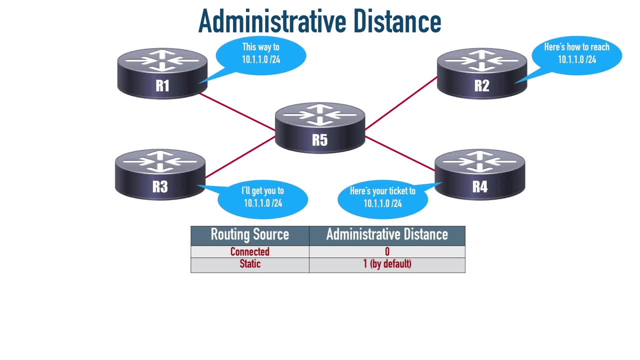 than the routing protocol we're using, And that route would kick in only if our routing protocol failed or the routing protocol could no longer get us to our destination network. Next we have internal EIGRP, And this is what we typically see in an EIGRP network, And it has an administrative 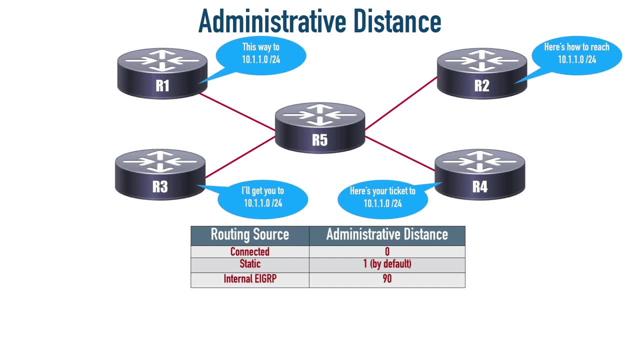 distance of a 90. Now I say internal because we're not redistributing those routes from an EIGRP autonomous system. Now let's go into another autonomous system like an OSPF autonomous system. Everything's happening within EIGRP. So it's internal EIGRP And it's got an AD of 90. OSPF is a little less believable. 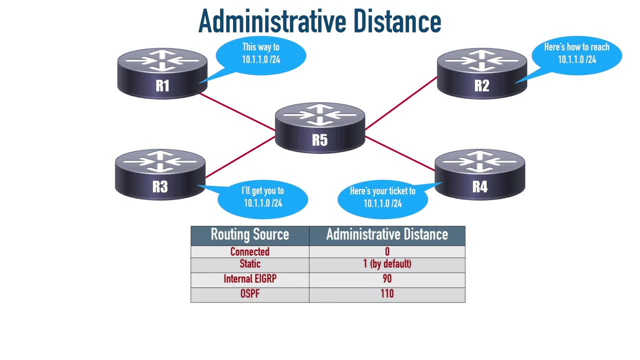 than EIGRP, with an AD of 110.. Behind that we have intermediate system to intermediate system with an AD of 115.. Then we've got RIP with an AD of 120.. And now let's talk about external EIGRP. It's much higher than internal EIGRP. 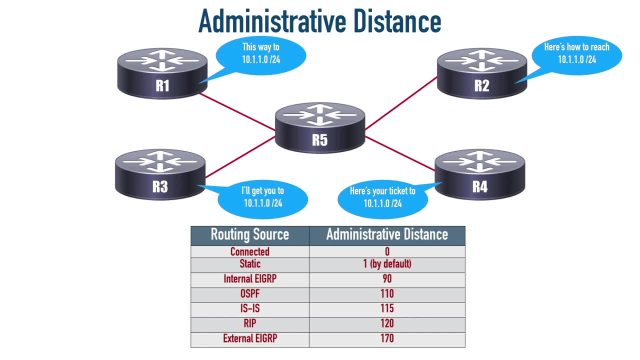 It's a whopping 170.. Now where would we see this? This is when we're redistributing an EIGRP learned route into another autonomous system. So if there's a network that EIGRP knows about and that route gets redistributed into, let's say, our autonomous system which is running OSPF, then that 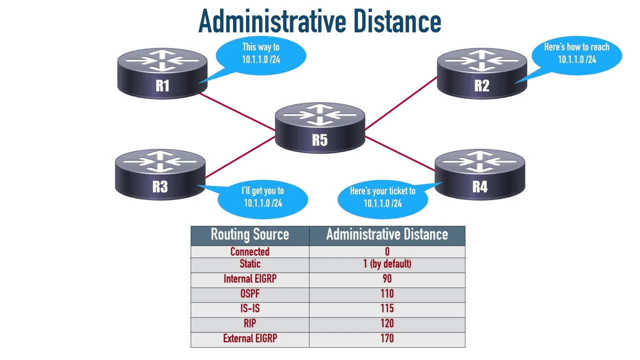 EIGRP learned route is going to have an AD of 170.. So even though OSPF is less believable than internal EIGRP, it's more believable than external EIGRP. Now let's go out to a live interface and take a look at administrative distance in action. 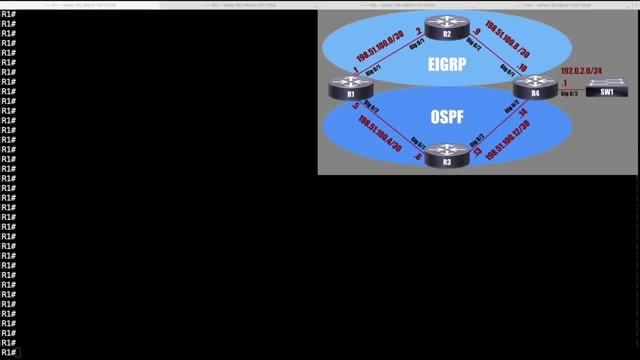 We're sitting here on router R1 and notice that R1 has its gigabit 0.1 interface running EIGRP and it's got its gigabit 0.2 interface running OSPF And both of its neighbors, its R2 neighbor running EIGRP and its R3 neighbor running OSPF. they are each telling R1,. 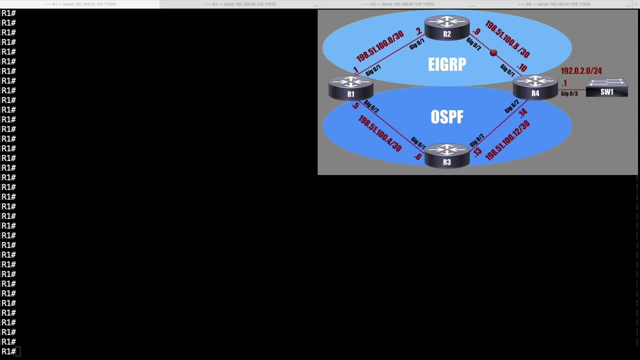 hey, here's how you get to the 192.0.2.024 network. That's the network hanging off of router R4.. In fact, let's prove that is indeed the case. Let's take a look at our EIGRP topology table. 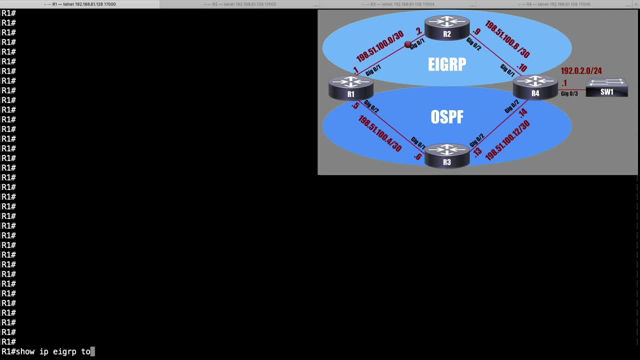 To do that, we say: show IP EIGRP topology And if we want to get to the 192.0.2.024 network, it says we should go to a next hop IP address of 198.51.100.2, and that's router R2.. 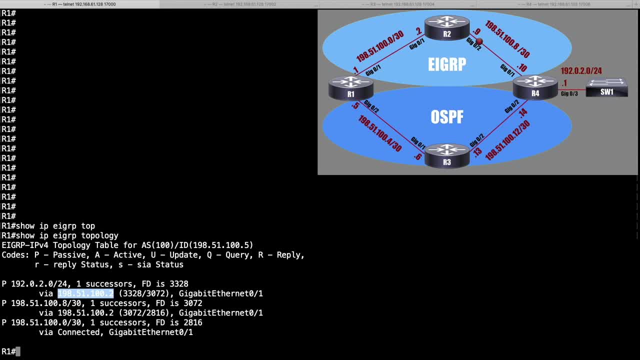 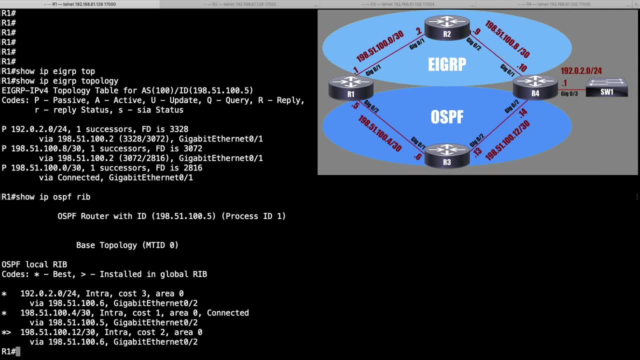 Let's take a look at OSPF's routing information base, or its RIB. We'll do a show IP OSPF RIB. Does it know how to get to 192.0.2.024?? It sure does. Here it is And it says we should go to. 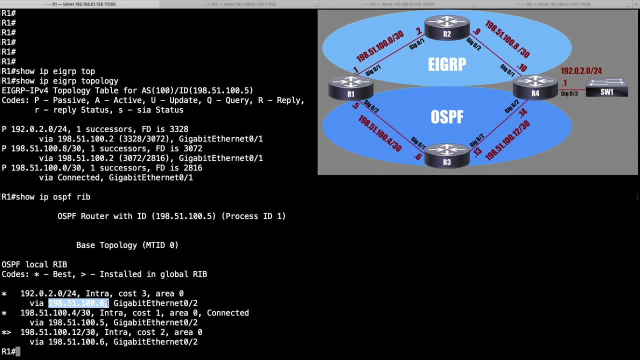 a next hop of 198.51.100.6.. That's R3.. They're telling R1 to go in different directions. So the question is: who does R1 believe? Well, it all comes down to the IP address of 192.0.2.024.2.. And, as we just discussed, EIGRP, specifically internal EIGRP. 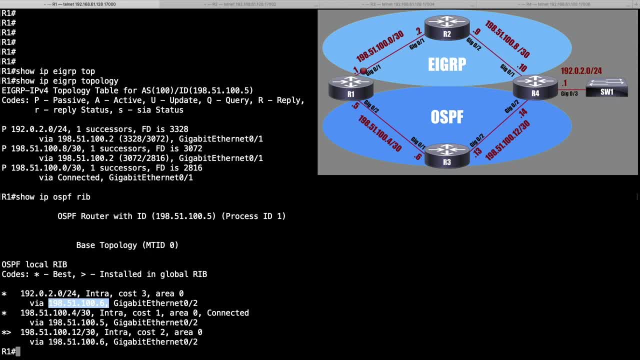 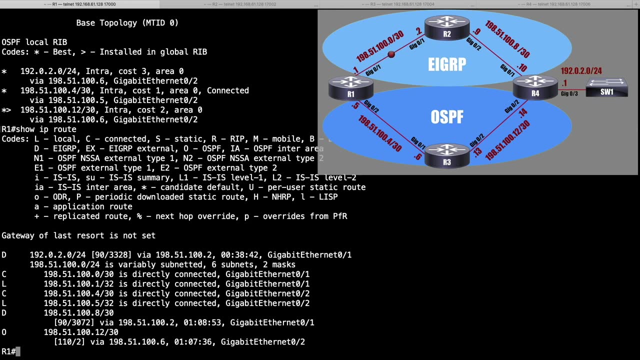 has a lower administrative distance than OSPF, which is 110.. Let's confirm that by looking at our IP routing table. Show IP route. And how does it think we get to 192.0.2.0.024?? Well, we know it was learned by EIGRP because we have that code of D. That means it was learned. the 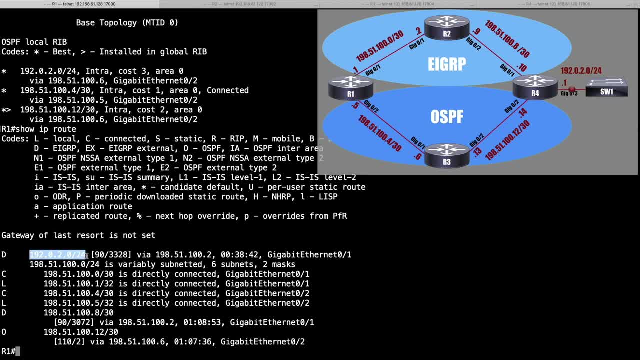 EIGRP And it says: if you want to get to this network, we're going to go to a next hop of 198.51.100.2.. That's R2.. And we also see evidence here of our administrative distances. 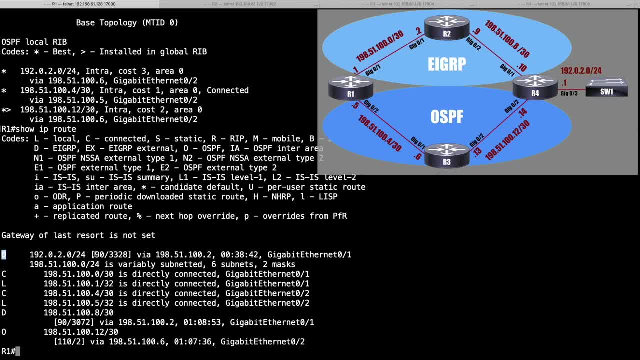 For the route that was learned via EIGRP. you see this 90? That's our administrative distance for EIGRP. And here's a different route for another network learned by OSPF. But notice the 110.. That tells us that the administrative distance for OSPF. 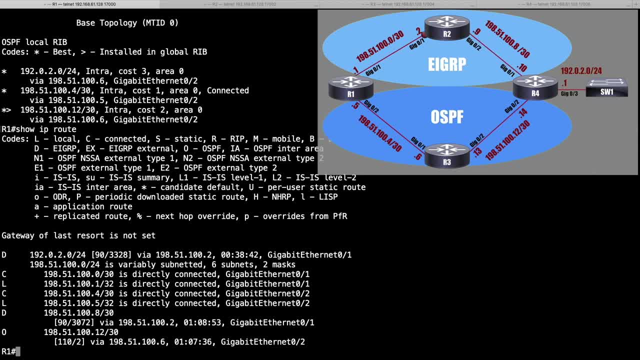 is 110.. So, since EIGRP had a lower administrative distance than OSPF, R1 believed EIGRP. However, as administrators, we have the ability to override that route, And one way to do that is to create a static route with a lower administrative distance. Now, 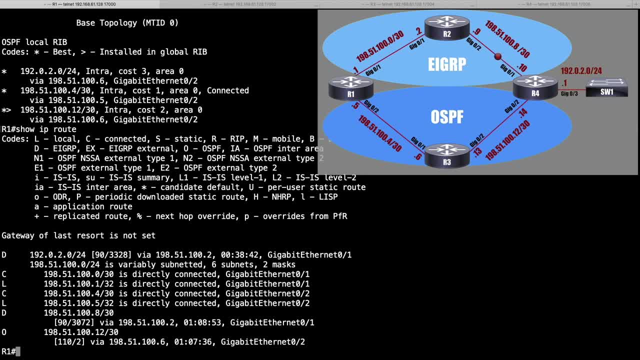 recall that, by default, a static route has an AD, an administrative distance of a one, Even though we can set it higher if we want to, if we want to do one of those floating static routes. But here let's override that EIGRP learned route by creating a static route To do. 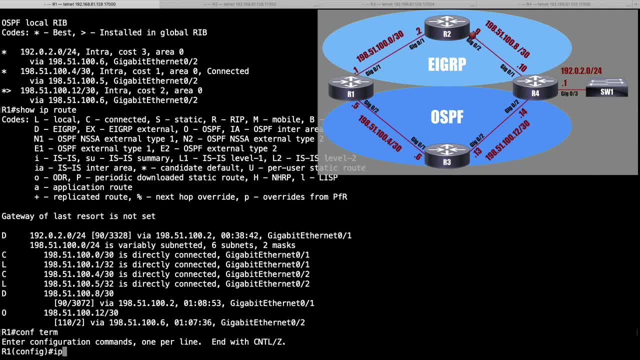 that we'll go into global configuration mode and I'll say IP route And I'm going to add a static entry for the network: 192.0.2.0.. And we're going to give a 24-bit subnet mask: 255.255.255.0.. 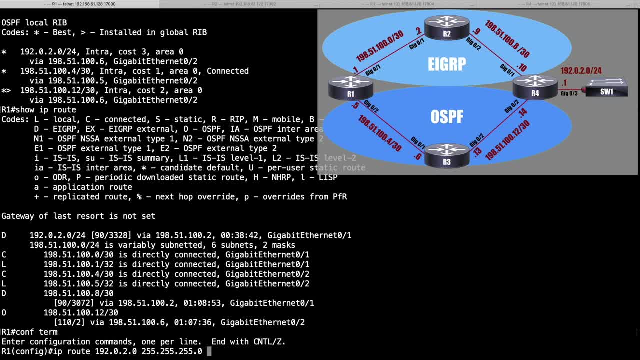 And now I'm going to specify the next hop. I want R1 to use, And let's say that I want R1 to use R3.. So I'll specify the next hop as 198.51.100.6.. That's R3.. Now, by the way, if I just pressed 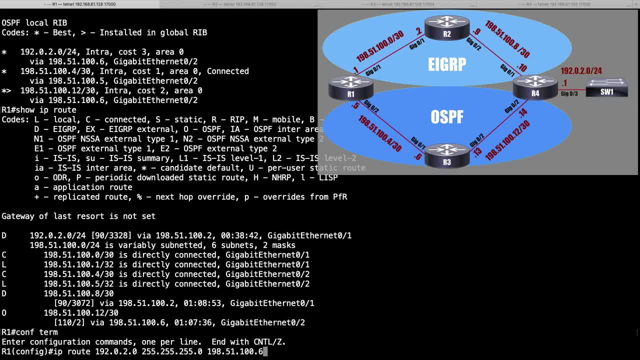 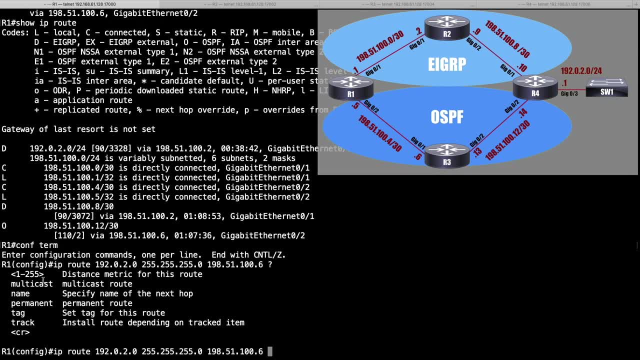 enter right now. that would set a static route with an AD of one. However, let's give some context-sensitive help. If I did want to set the AD to a higher value, here's where I could do that. I could set it anywhere in the range of one through 255, but we're just going to stick.